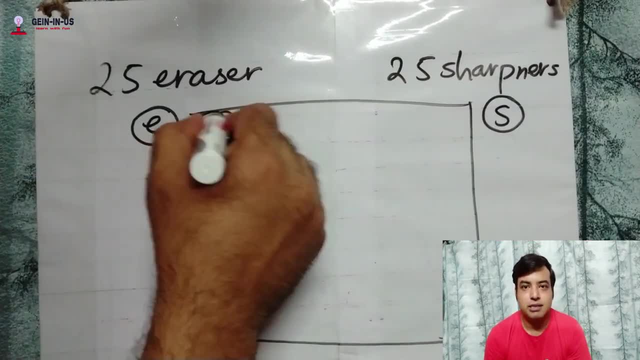 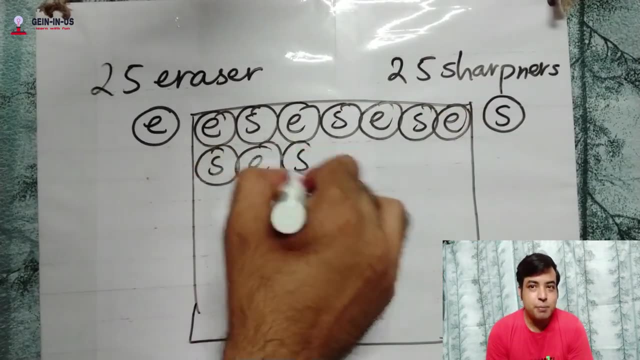 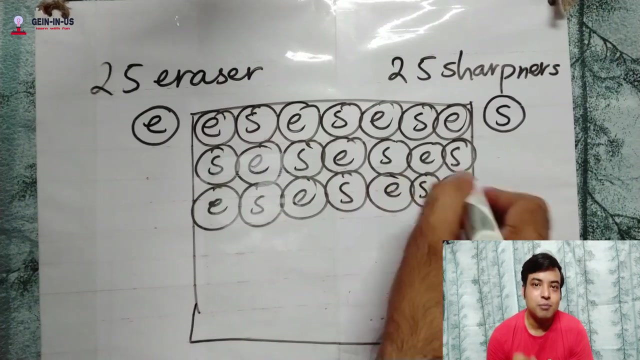 sharpener. Okay, So we are mixing the eraser and sharpener together, Okay, And now you can see that how they are mixed. If you take out any part of this box, then what we will find, We will find that both eraser and sharpener will come together. Okay, In a definite proportion. 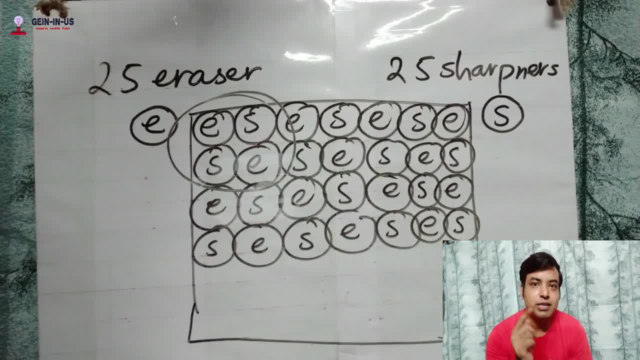 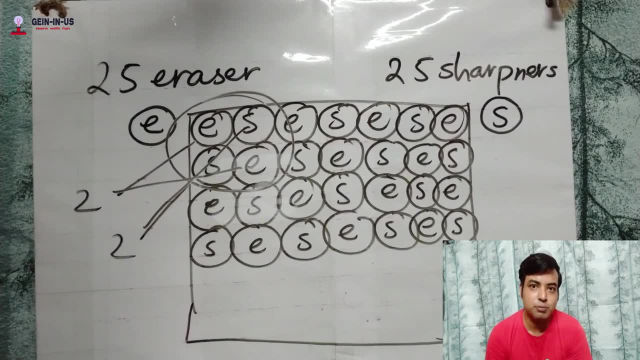 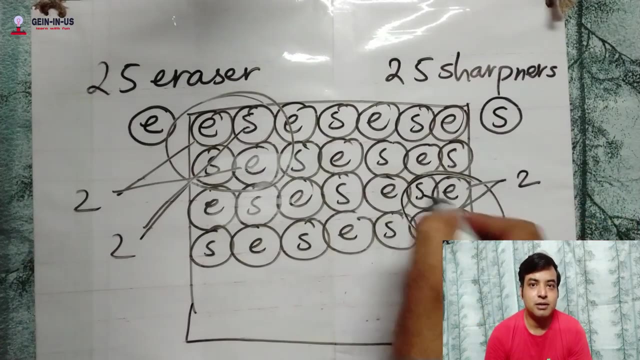 E and S. this portion I have taken Here, two E and two S are there. That means two eraser and two sharpener. Okay, The same portion. if I take it from other portion, other part of this box, Okay, There also I will get two eraser and two sharpener. If any other. 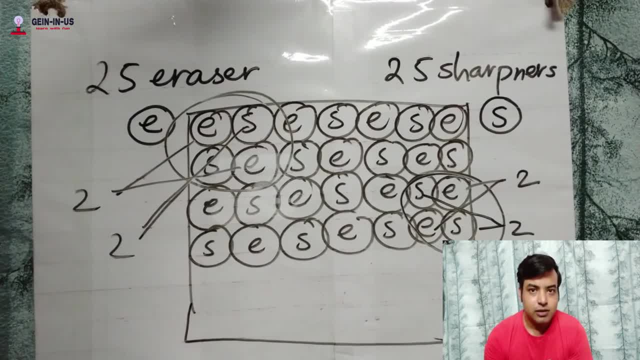 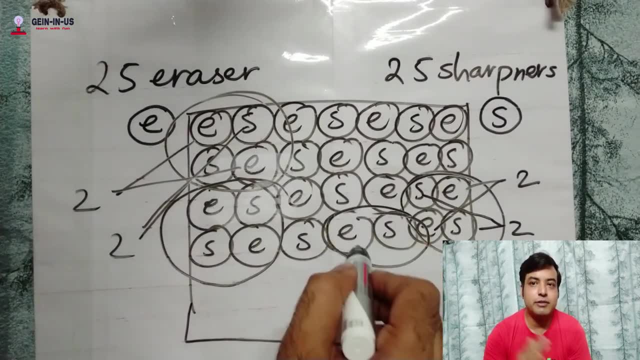 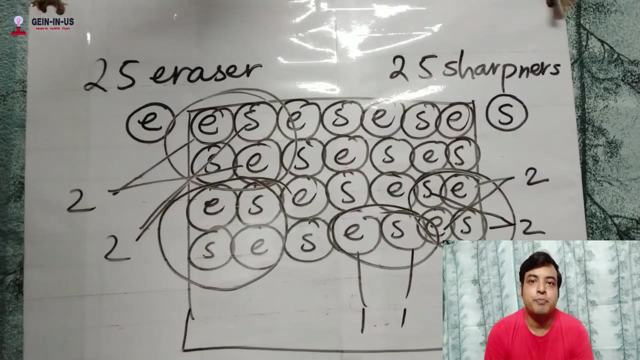 portion. if I take, okay, there also, you will get two eraser and two sharpener. Okay, If I reduce the amount, then I will get one eraser and one sharpener. Okay, That means we are in a same proportion. Okay, Wherever I will take, I will get the same proportion, Okay. 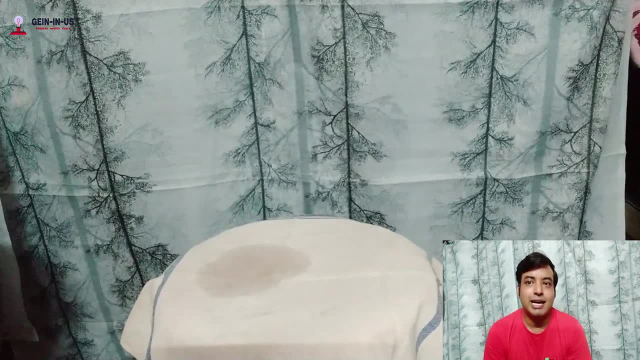 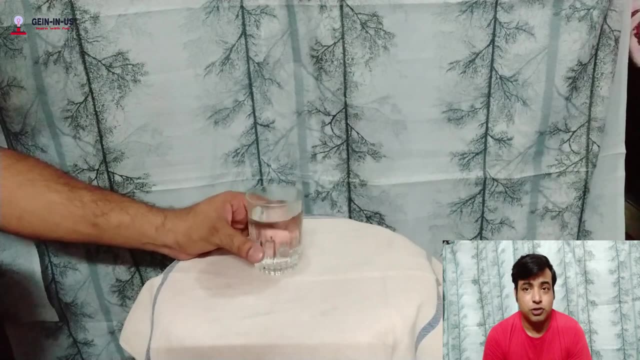 Same is the case of: okay, if I take a glass of water, Okay, And I add salt in it. Let's take another example. Okay, For that we need one glass. glass of water, Okay, Water is also needed, and little amount of salt. You can see the salt. Okay, Now I will add one. 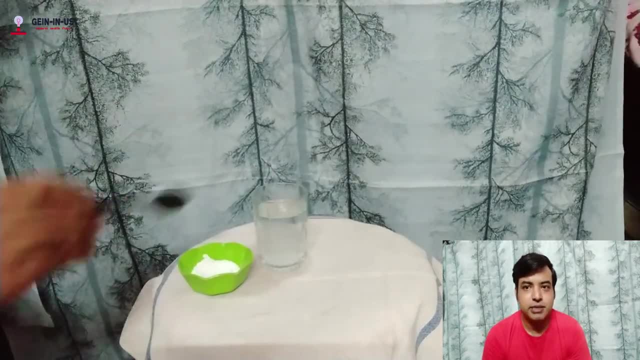 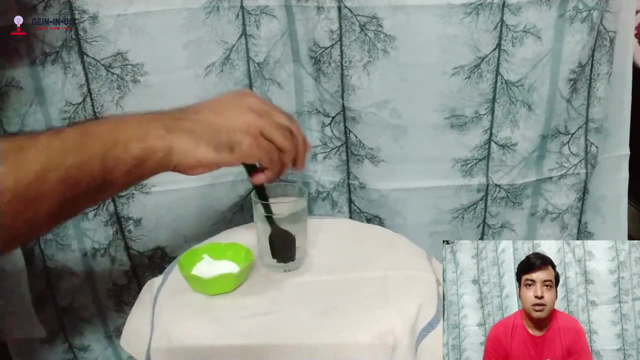 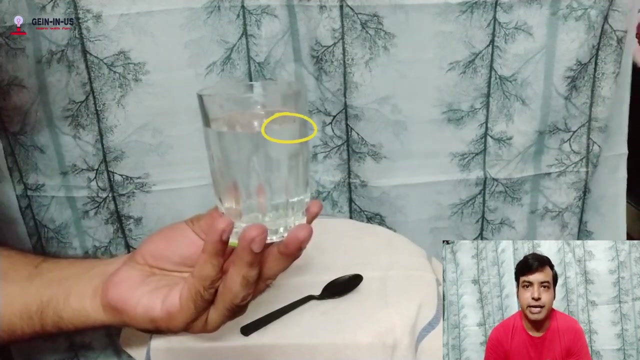 spoon of salt into this water, Okay. And then mix it: Okay, You can try it at your home, Okay. And now, from this glass of salt water, Okay, What you will find? Okay, If you take this portion of water, or this portion of water, or this portion of water, any portion of water, 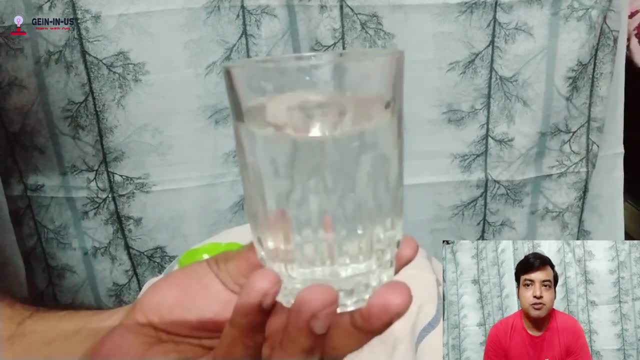 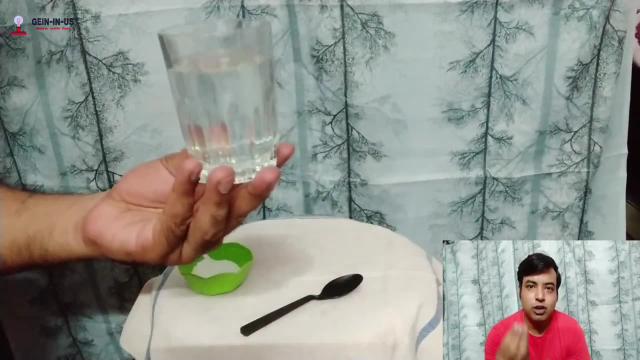 if you take, then what you will find? you will find the same amount of salt. Okay, You will find it salty. If you taste it, you will find it salty. Okay, Why it is salty? Because the salt is present thoroughly in this water. Okay, It is distributed equally in every parts. 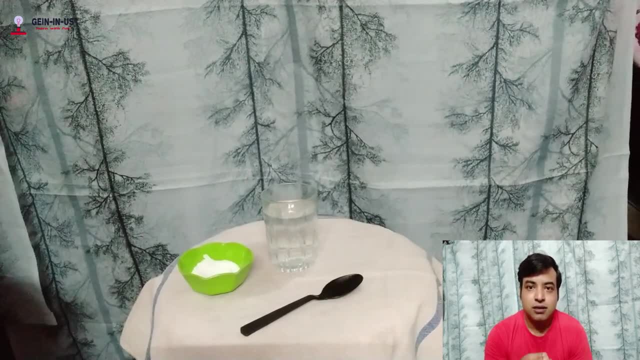 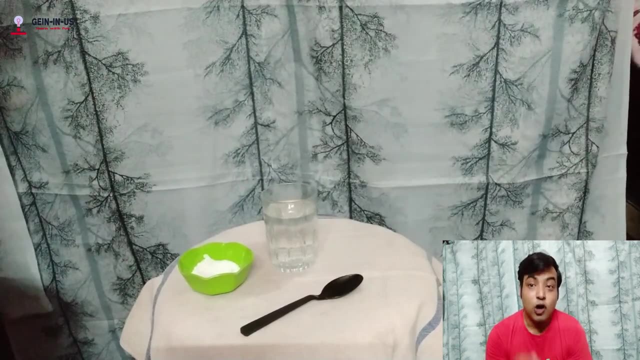 of the water. Okay, So that's why it is salty. Okay, And now, from this glass of salt water, you can see that salt is present thoroughly in this water. okay, This is the espacio, and the battle in that glass of salt water is friction. Okay, Let's take another example from this. 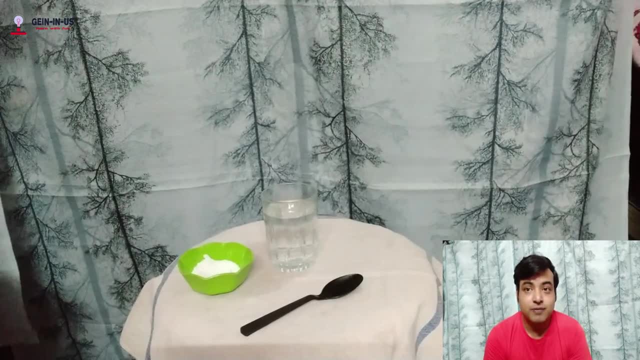 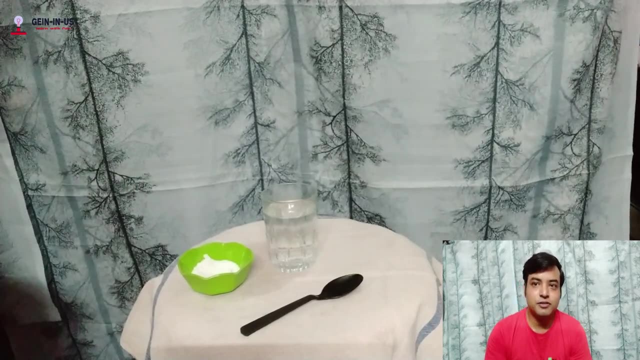 water. So this water already is in the mixture. Okay, This is the biological mass of it and it already is death in it. Okay, This is the incubation заключed in the mixture, in the material body. So what you will find is that? okay. So I need right from that, I just need 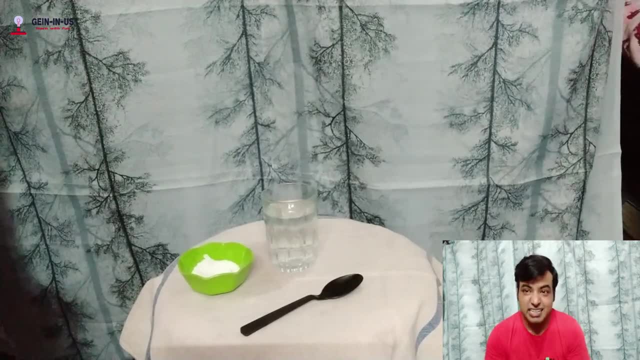 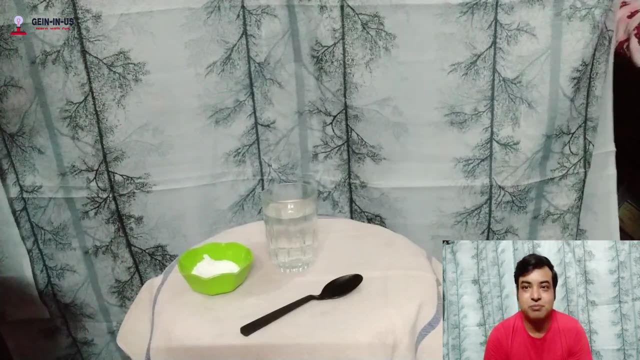 two different types products. One is: think of all the smells. that is not something that would be applied after. let me show you one of them, Okay, And then from that drink you mixture. okay, now, if i take this previous example, rubber and sharpener if i mix them together. 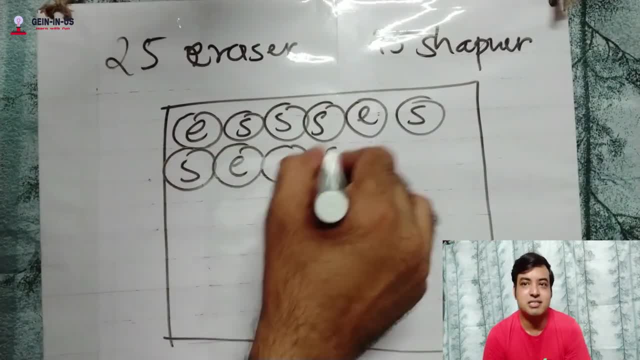 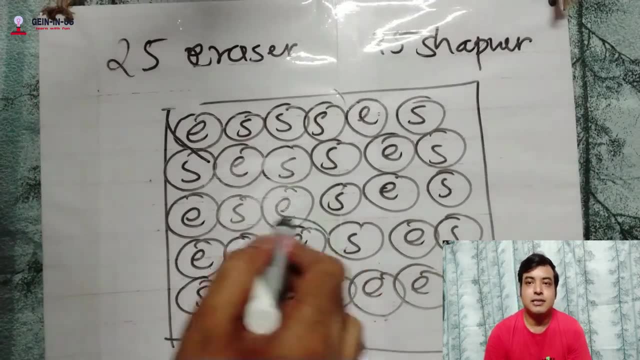 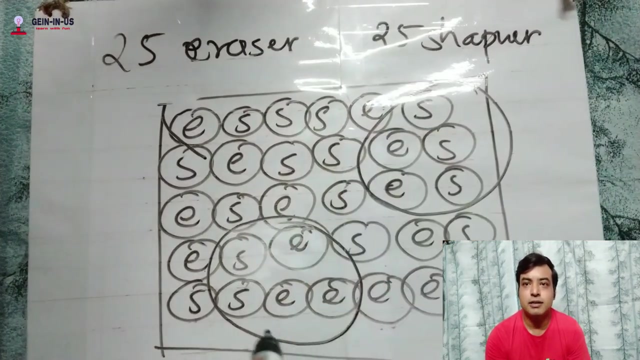 then you will find that if i mix them haphazardly, randomly, if i mix them- okay, now, i'm mixing them randomly, okay, now, from this portion, if i collect, then here you will find three erasers, two sharpeners. okay, if i collect it from this portion, then you will find two eraser, three sharpener. okay, 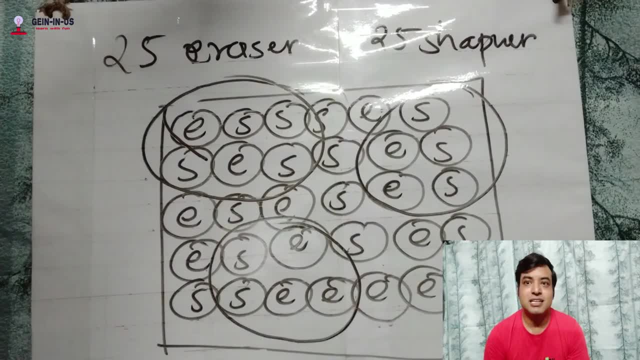 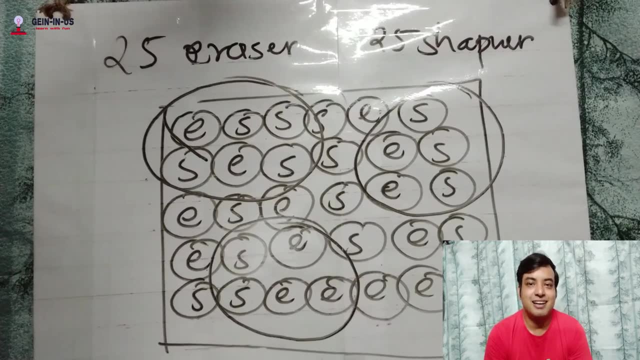 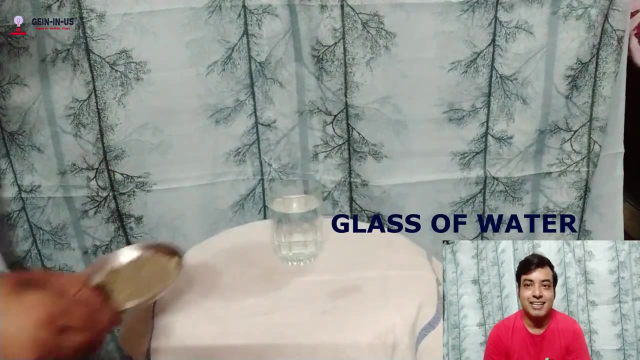 one eraser, five sharpener, okay, like this. different, different proportion. you are getting not the same, not the equal thing. you are getting okay, and this type of mixture is known as heterogeneous mixer, like, if i take an example, another example: for that also, we need a glass water, okay, and then i 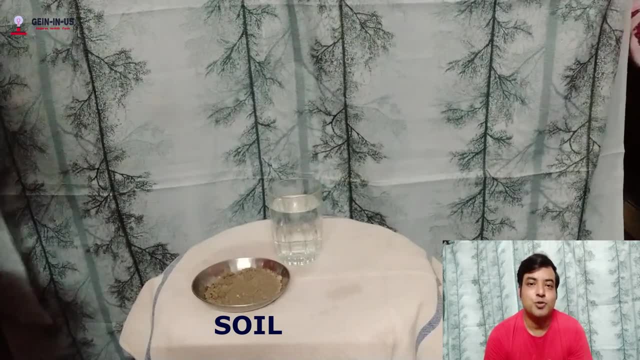 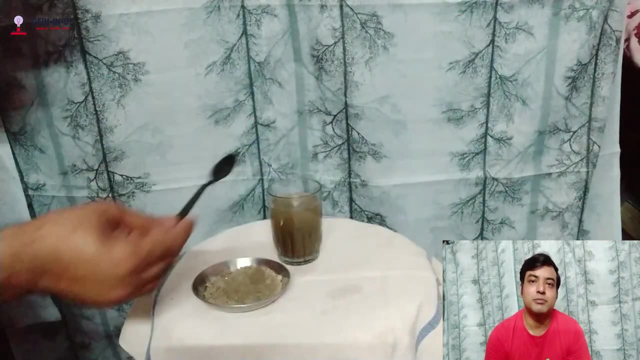 have to add soil. okay, so what you will get if i add soil, then it will mix the soil. the heavier particles will settle down at the bottom, the lighter particles will mix in the water. Okay, Then, from the bottom, if you take out the water, then you will find more. 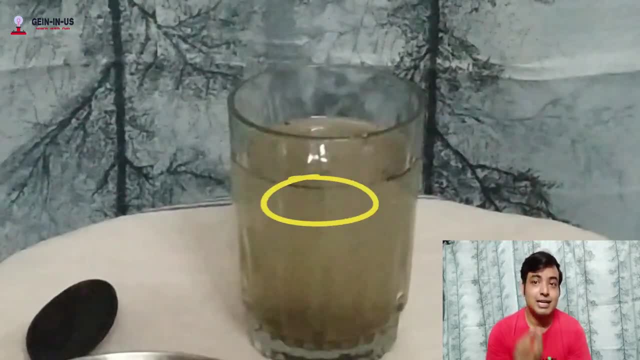 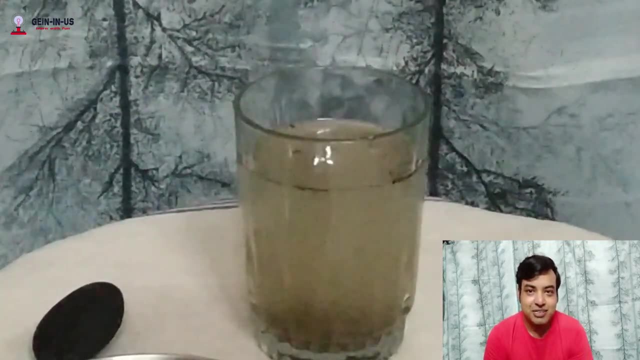 more soil particles. Okay, From the above, if you take out water, then you will find less soil particles. Okay, So that means the soil is unevenly distributed in the water. Okay, That type of mixture is known as heterogeneous mixture. So have you understood what is mixture? 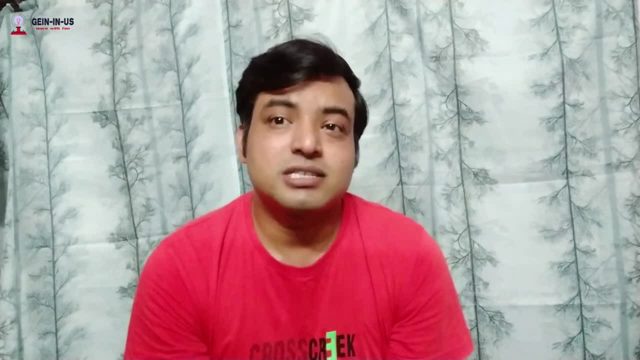 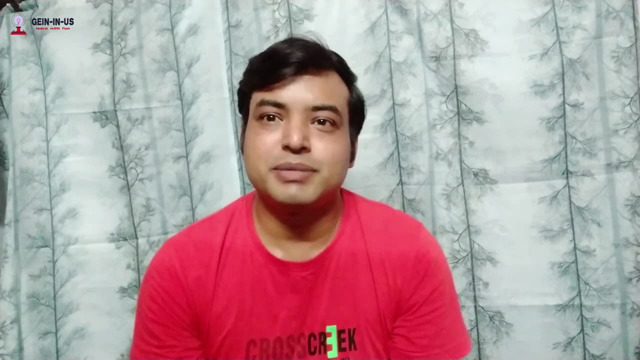 Homogeneous and heterogeneous mixture, Okay. Okay, We can mix two things together. Okay, Like we know matter: solid liquid and gas. Okay, This type of substance, we can mix them together. mix and match: Okay, We can make different kinds of mixtures. Okay, Like if I make mixture of 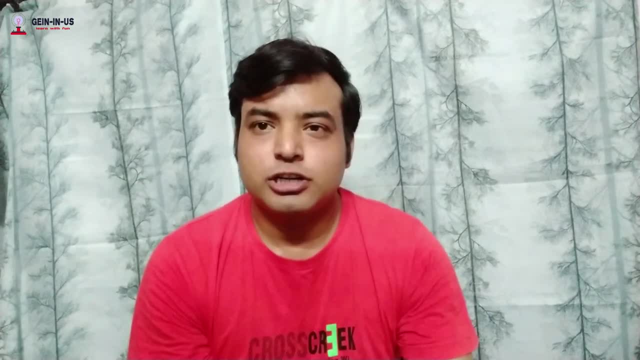 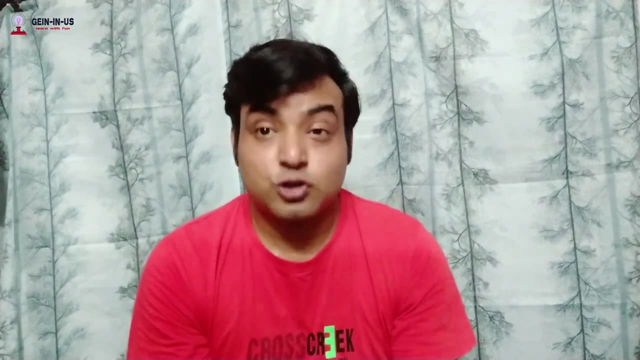 solid and solid: Okay, Solid and solid- two types of mixture we can make. One is homogeneous, one is heterogeneous. If I talk about homogeneous mixture of solid and solid substance, Okay. If I take two solid substance together, Okay. And mix them in a homogeneous way: Okay. 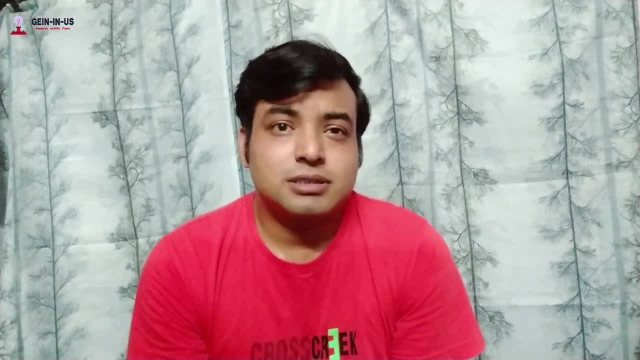 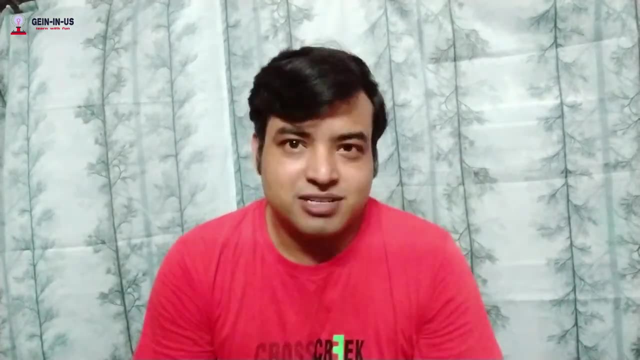 Then what you will get. Okay, So you have come across the term known as alloys. So if you talk about alloy, alloy is the homogeneous Mixture of two solid substance. Okay, So let me take the example of an alloy. Okay, That is brass. 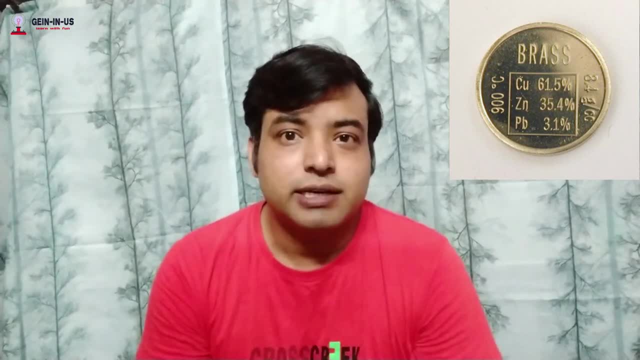 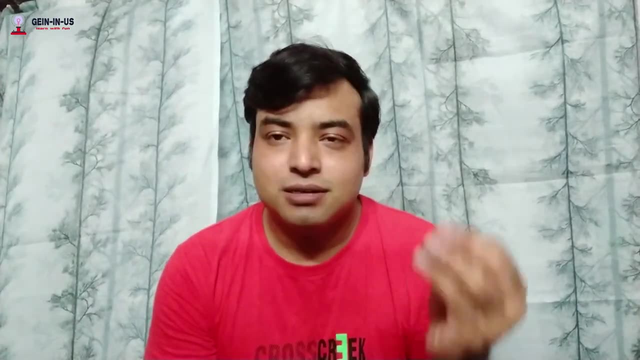 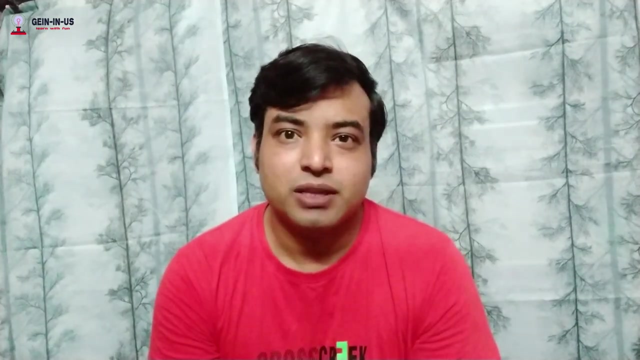 Brass is made up of two substance: copper and zinc. Okay, So it is a mixture, not the compound. Okay, It is not chemically mixed together. Okay, So brass is an alloy of copper and zinc. Okay, When copper and zinc mix together in a homogeneous way. Okay, Make a homogeneous mixture, Then it. 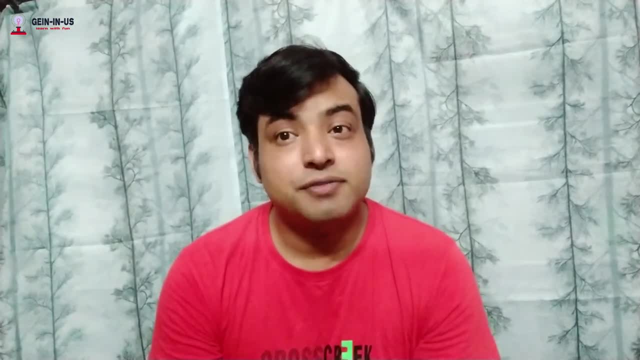 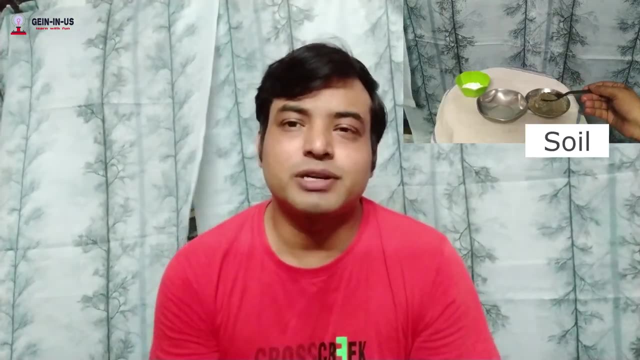 makes an alloy of alloy known as brass. Okay. Likewise, if I talk about a heterogeneous mixture of solid and solid substance, Okay, You take salt and soil and mix them together. Okay, It will become a heterogeneous mixture of two solid substance. 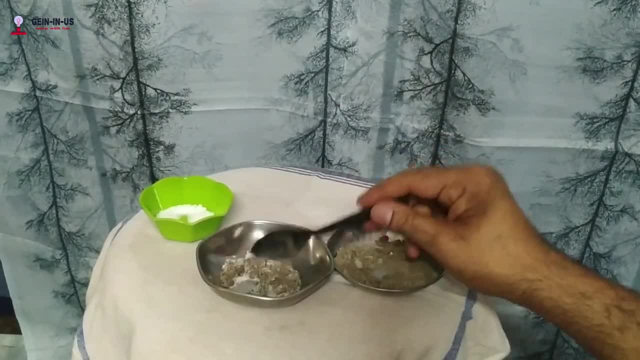 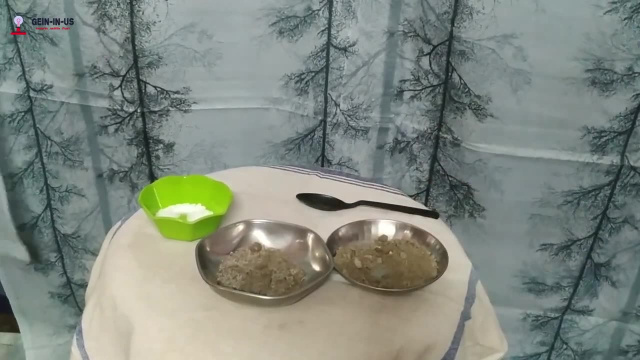 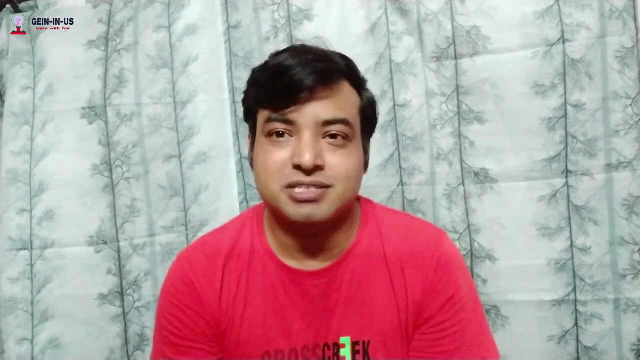 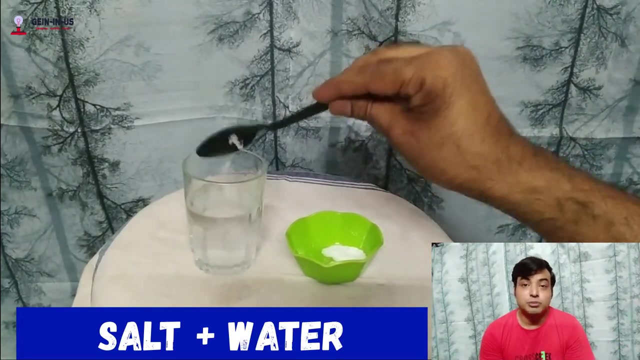 Okay, Now, if I talk about mixture of solid and liquid, Homogeneous mixture and heterogeneous mixture, already I have shown you: if you mix two substance, one is solid and one is liquid, like water and salt- when you mix together, ok, then it will become a homogeneous mixture of two substance. 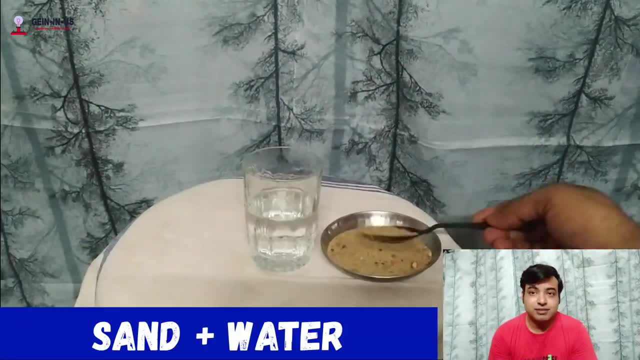 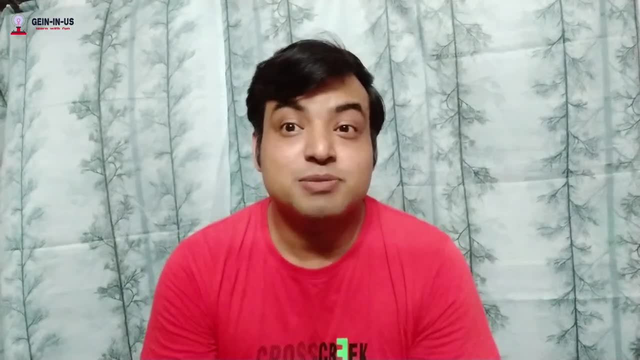 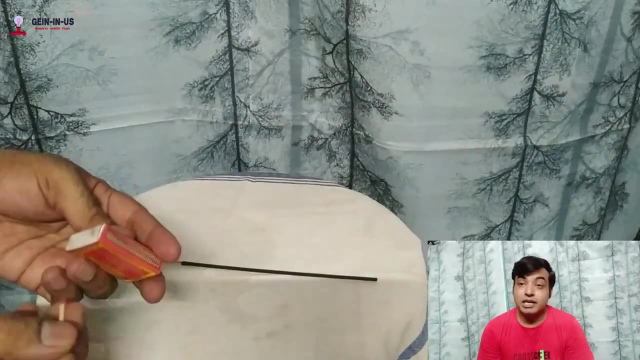 of solid and liquid: ok, if you mix water and sand, ok, it will become a heterogeneous mixture of solid and liquid. now, if I talk about mixture of solid and gas, smoke is the mixture of solid and gas. now you can see. I have scented sticks. ok, if you burn the scented sticks from the 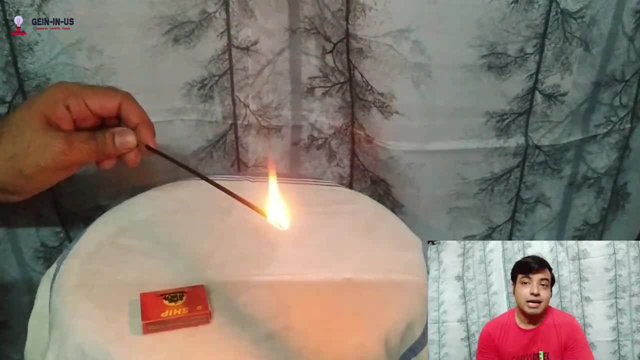 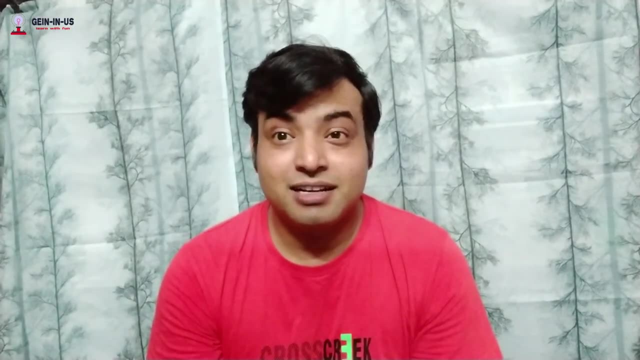 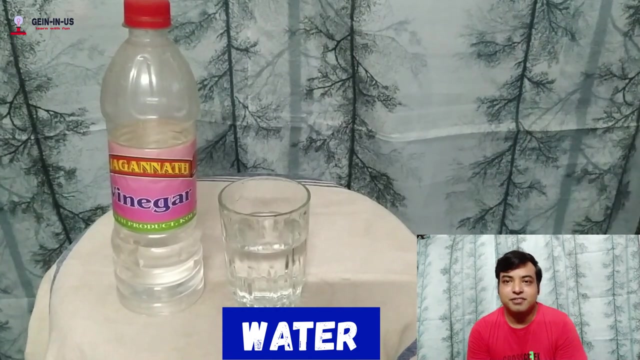 scented sticks. some smokes are coming out. ok, these smokes are the mixture of solid and gaseous particles. ok, now, if I talk about liquid and liquid, mixture of liquid and liquid, ok, now I have two substance, two liquids. ok, one is water, another is vinegar. ok, vinegar is. 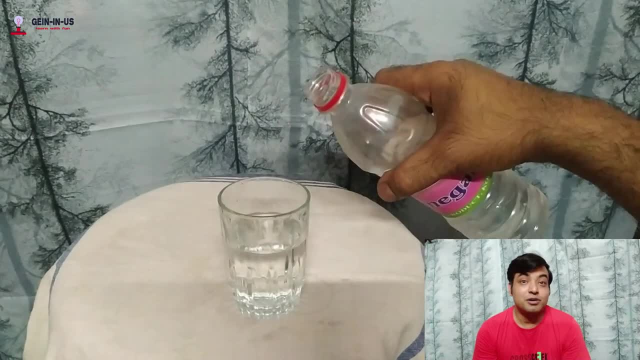 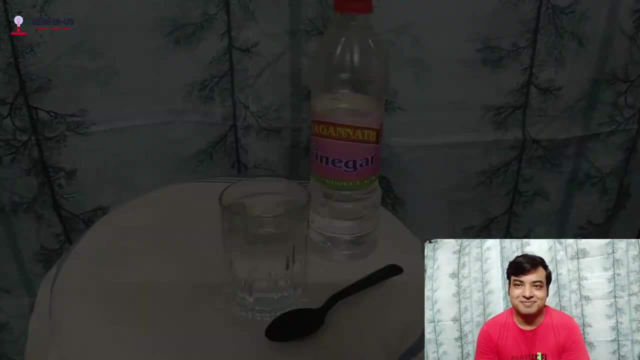 a liquid which we use for cooking purpose? ok, So now, if we add Vinegar into the water, ok, now mix it thoroughly. you will find it. it has become a mixture and it has become a homogeneous mixture. now, if I talk about mixture of liquid and gas, I will 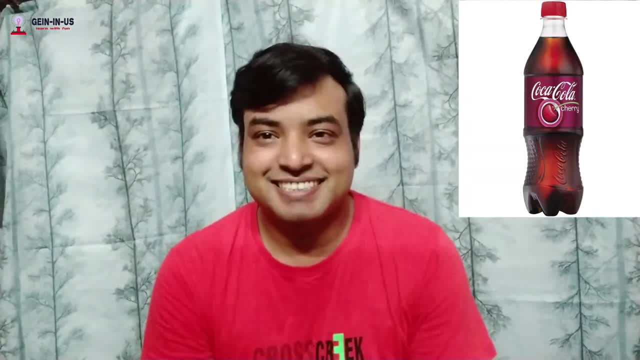 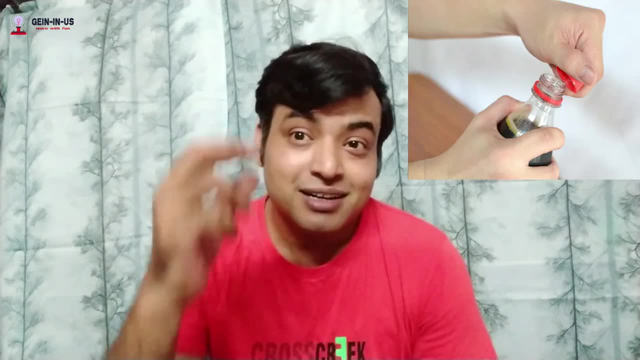 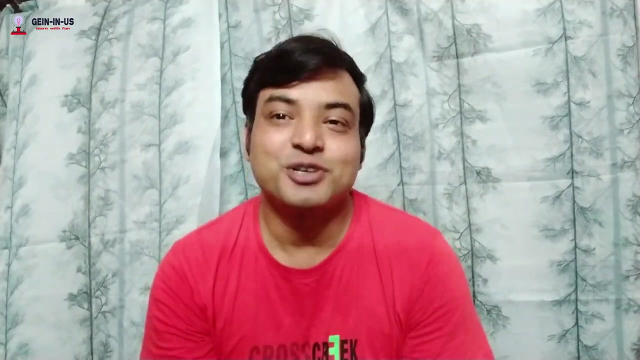 find mixture of liquid and gas. see this. what do you find it out? this is coca cola or pepsi, you can say. ok, when you open the bottle, what you find? some gas is coming out. why it is so? because that gas is mixed in the water. ok, so it is a mixture of liquid and gas. ok, 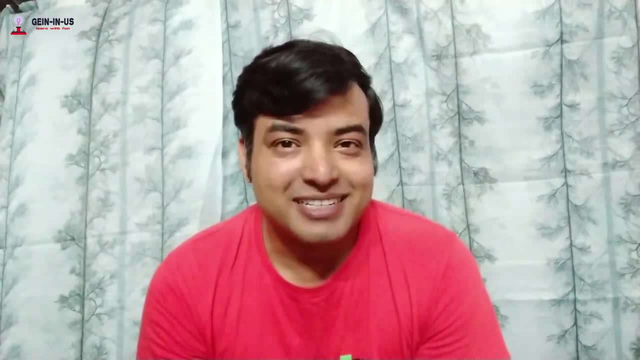 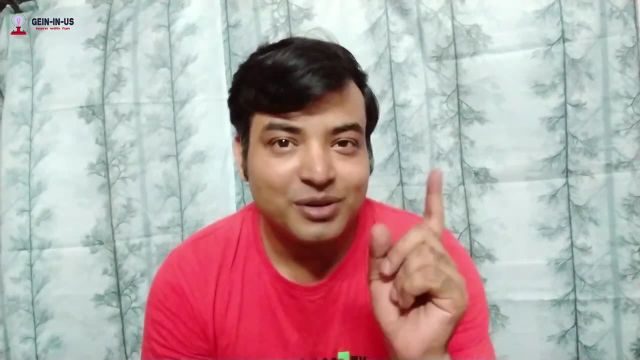 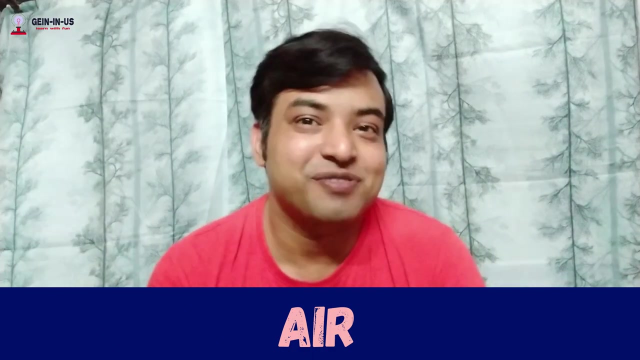 now, if you talk about mixture of two gaseous substance, what is that? can you tell me, mixture of two or more gaseous substance? ok, definitely, I know that. you know it. ok, what is that it is? yeah, that is what we are present. ok, it is a mixture of many different kinds of gas. 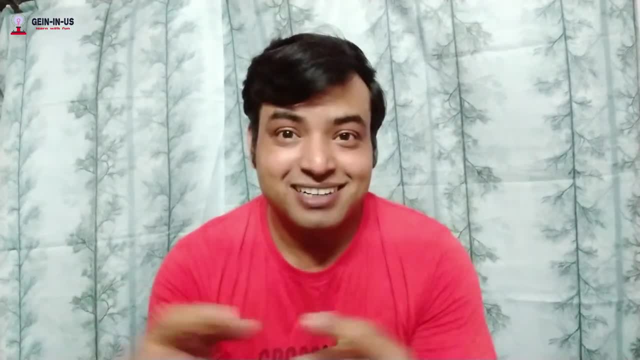 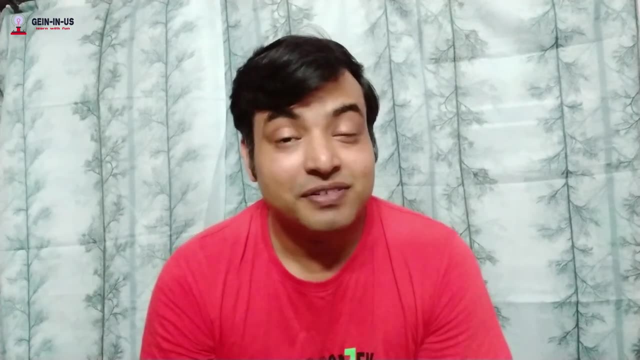 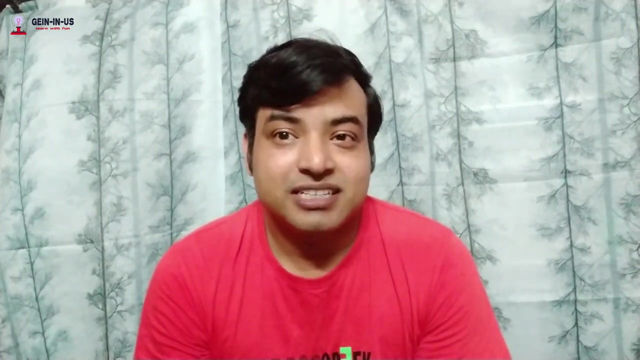 ok, so this is a mixture of gas. this is not the. this is: they are not chemically mixed, they are physically mixed together. ok, and this mixture can be separated by means of physical methods. Ok, so this is all about mixtures. ok, now, if you talk about solution, ok, solution means 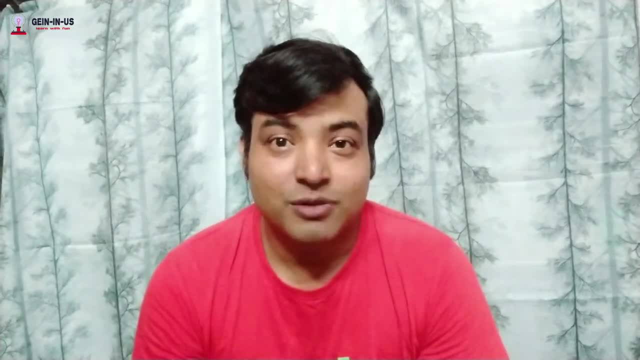 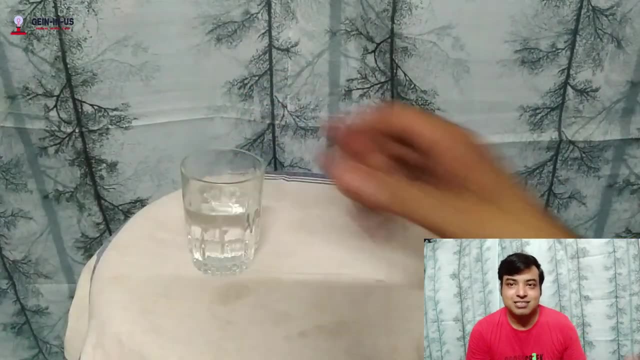 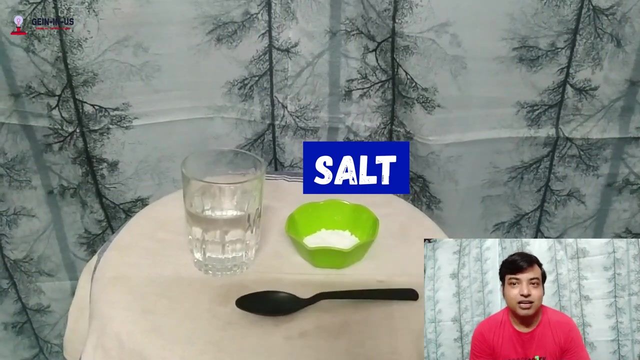 what when two substance dissolve together? ok, one substance is known as solute, another substance is known as solvent. ok, now I have a glass and I have taken one solvent. that solvent is known as water. ok, and I have taken this. this is salt. this is known as solute. ok, 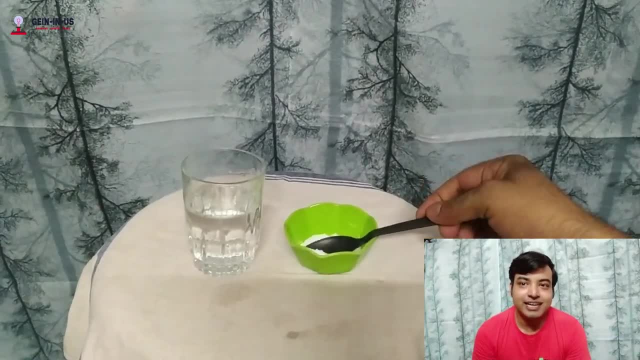 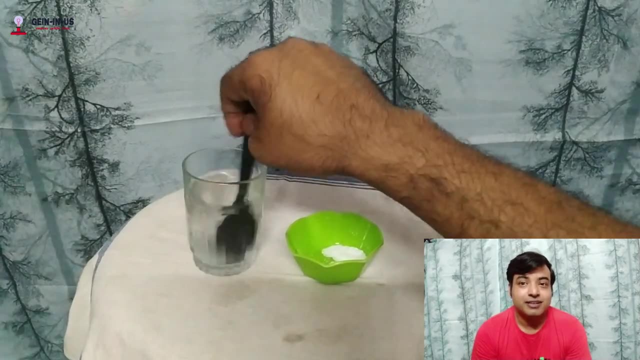 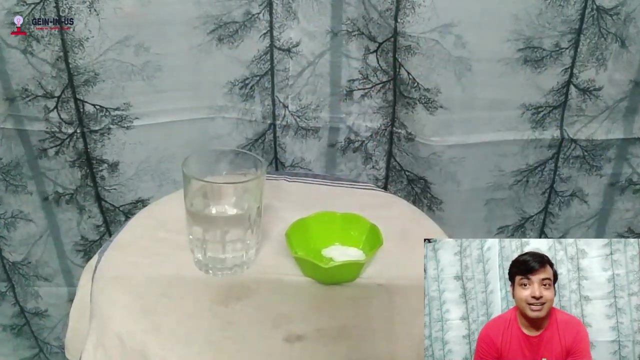 now, if we add this solute in this solvent and I will stir it ok, Ok, It will mixed. so, after mixing what you will find, you will, you will find a solution of salt and water. so this is the solution of salt and water. ok, where water is the solvent. 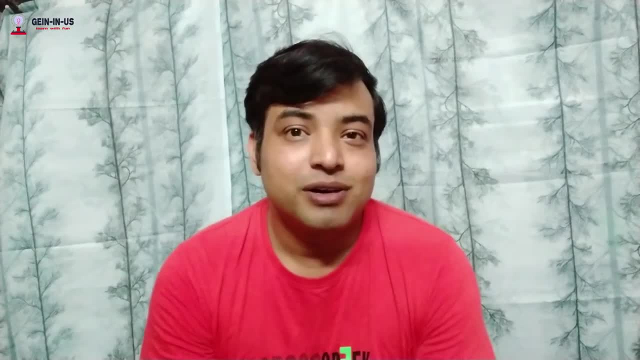 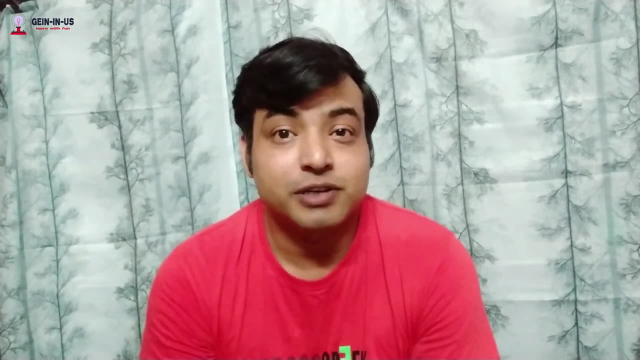 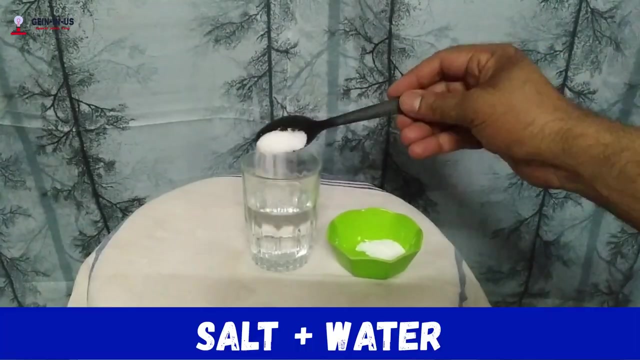 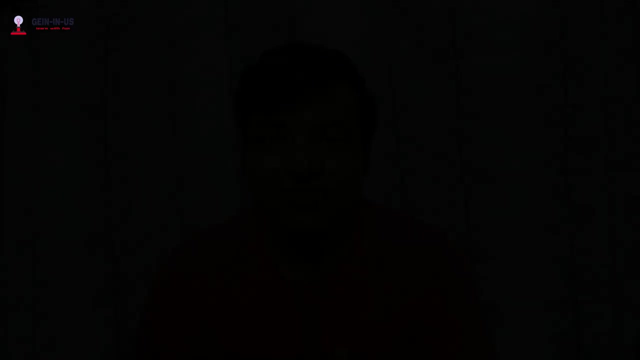 and salt is the solute. ok, now we can make many solutions like that. ok, in water. so that is why water is known as the universal solvent. why? because water can dissolve many substance, like salt, Ok, Like any sugar, Ok, Yes, Like true, like promise, which contain all elements of human substance. right, 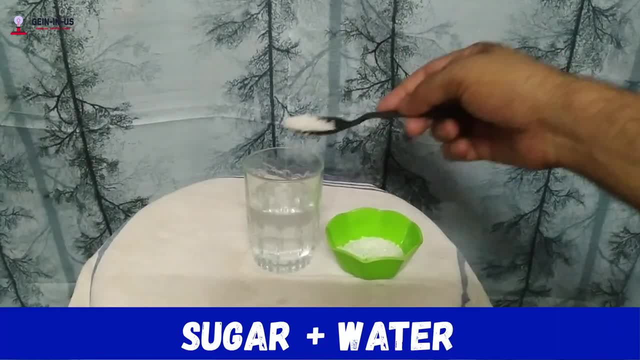 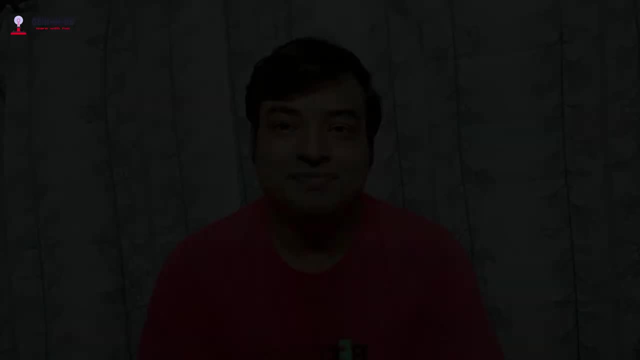 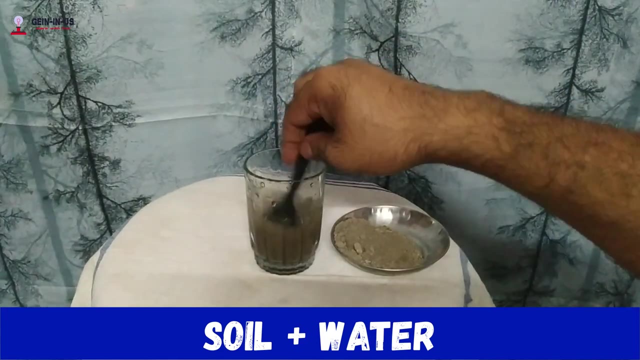 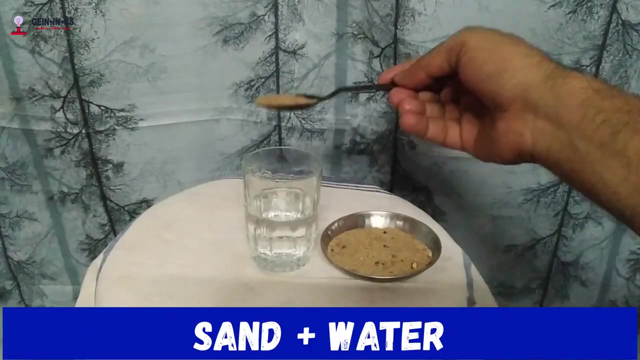 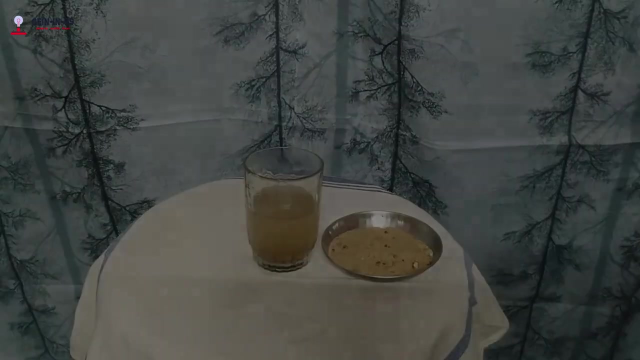 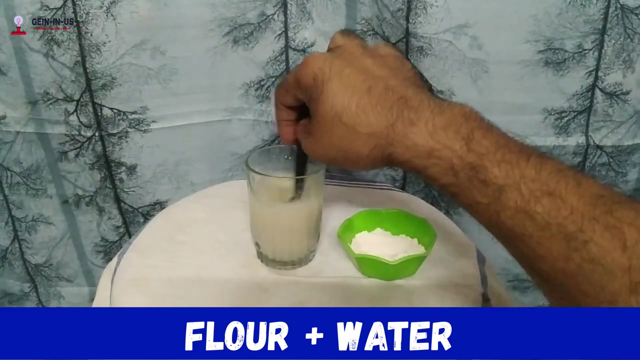 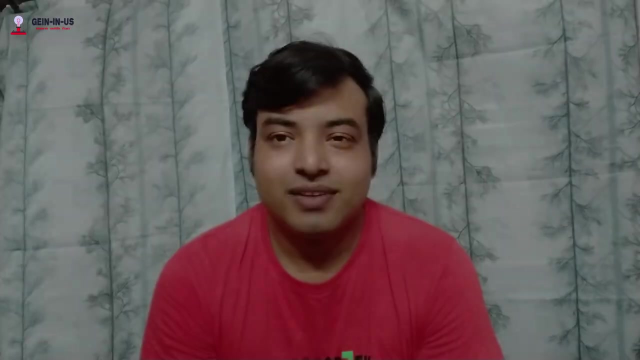 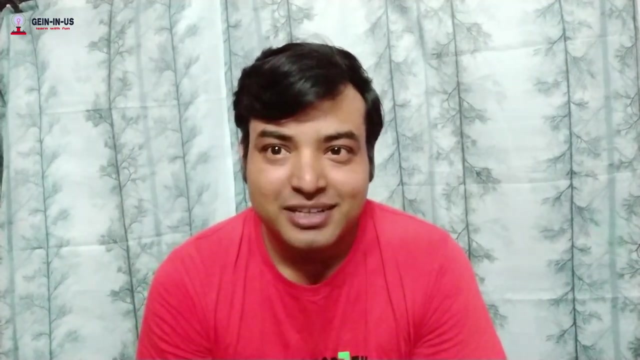 Like sugar, Yes. Like soil, Yes. Like drop, Yes, Yes, Yes. sand like floor. So many substance can be dissolved in water. that that's why water is known as the universal solvent. Okay, When two substance- solute and solvent- mix together, they are known as solution.